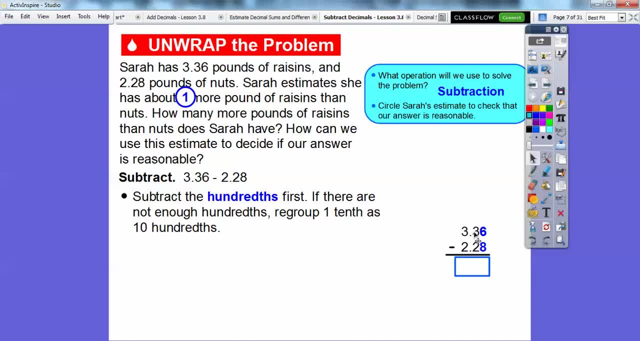 And if there's not enough hundredths, we're going to regroup the tens. So these three tens, we're going to regroup and borrow from one another. So we're going to take one of these three tens and make it a two ten, and then that borrowed ten is going to go over here and make this sixteen hundredths. So there we go right there. So this three became a two and this six becomes a sixteen because we added ten hundredths to it. okay, 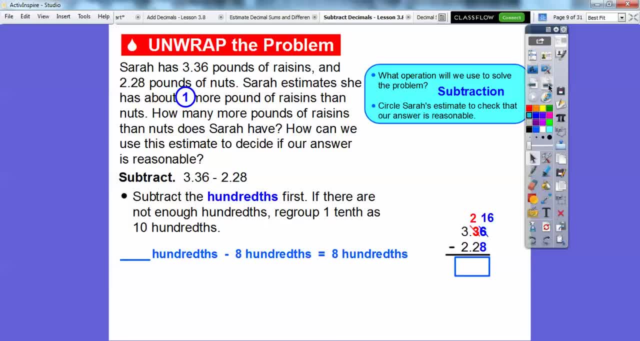 All right, and then we can subtract the hundredths right there. So sixteen hundredths minus eight hundredths gets us this eight hundredths right here. okay, All right, let's slide that up. We're running out of room here, So okay, now let's subtract the tens, okay. 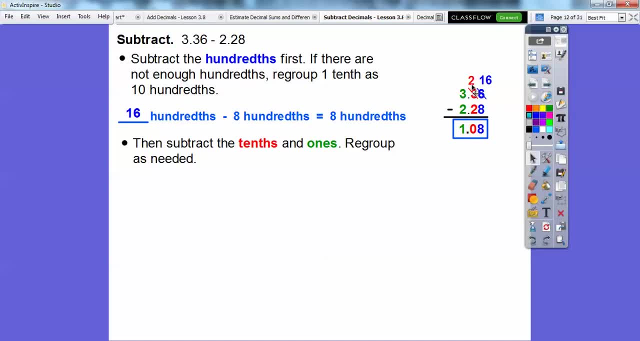 So and the ones. So when we subtract the tens, it's now: two tens minus two tens is zero. and then three ones minus a tenth. sorry, two tenths minus two tenths is zero tenths. and then three ones minus two ones is one one. right there, okay. 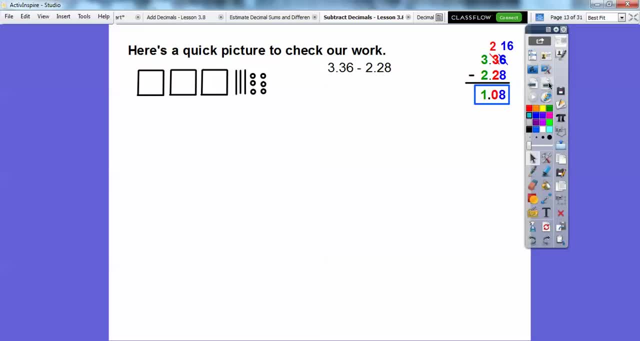 So the answer is 1.08, okay, Here's a quick picture that would check our work on that. okay, So we know the answer is 1.08.. All right, so here's 3.36,. okay, Remember, these are ones, these are tenths. 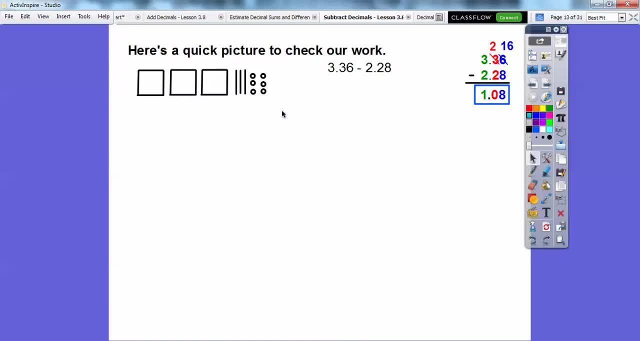 And these are hundredths right here. So here's 3.36.. Okay, now, before we subtract this hundredth off, we need to regroup, okay. So we're going to regroup this tenth right here and make it ten hundredths right here. 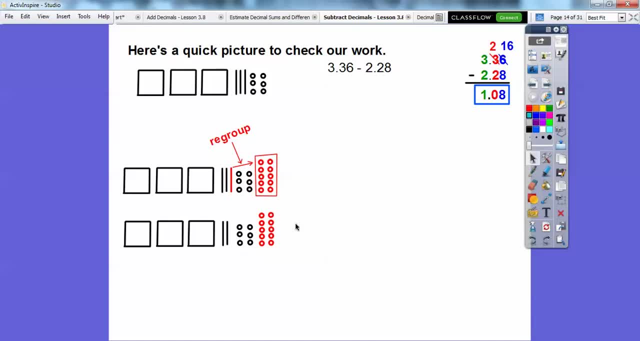 So I took that away right here, And so now this is the same right here as this. We haven't borrowed that. Now we're going to subtract those, these 8 hundredths right here. When we subtract those 8 hundredths, it took out eight of these right here. So took out these six and then these two, These six, and then two eight hundredths. right here, Right now it just looks like 100.. Okay, 5 ,0.. This is correct, So we got it right here, which is all right here. So small, this regretted a small decrease in time, and now it's ten hundredths plus theHundredths. 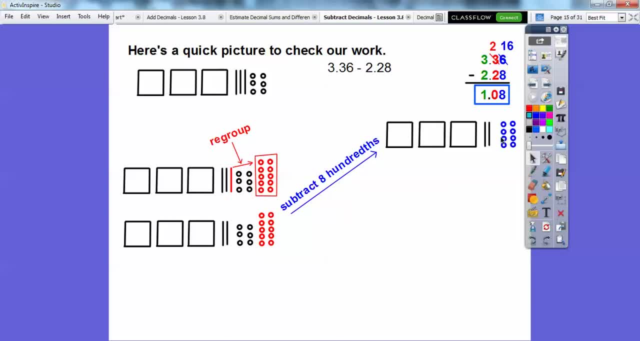 two right here, okay, so we still have the eight right there, okay. and then now we're going to go ahead and subtract, subtract these two tens. so we're going to subtract these two tens right off right there, so those aren't there anymore. then we're going to subtract these two ones next, you guys. so when we 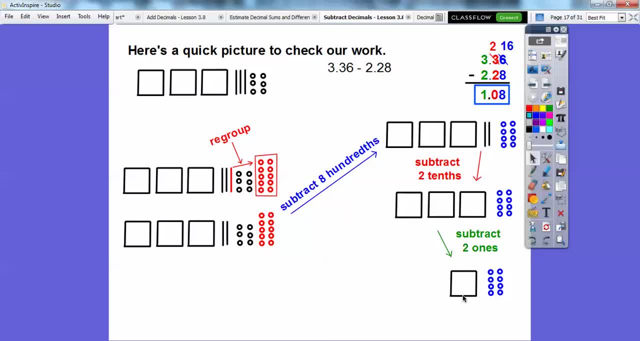 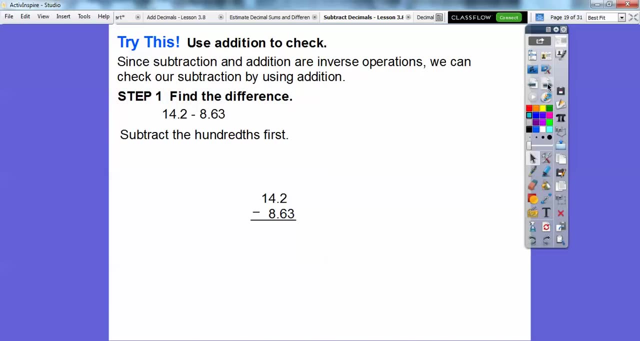 subtract those two ones. there's our answer right there. this is one and we don't have any tenths left, so that would be zero tenths and then eight hundred. so one point zero eight, right there, okay, all right, pretty cool, huh? okay, let's try this, you guys. since subtraction and addition are inverse operations, we can. 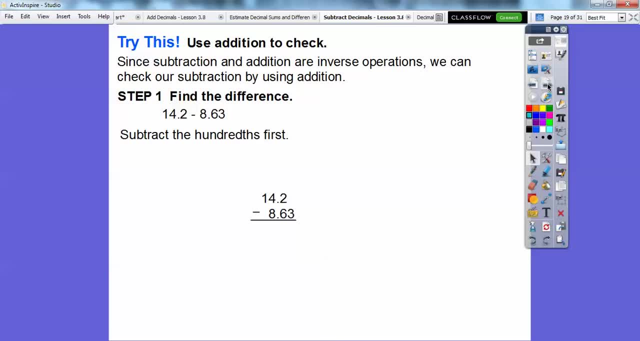 check our subtraction by using addition. so let's try that with this one. fourteen point two minus eight point six, three. so first we're going to subtract the hundredth, so we need to include that zero right there. fourteen point two is the same as fourteen point two, zero. okay, then we got to borrow from this two. 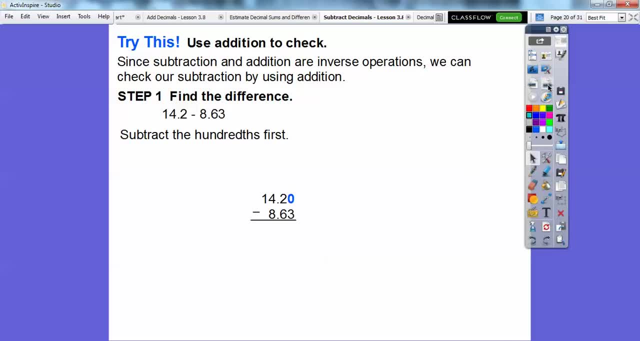 tenths right here. we're going to make it one tenth and make this ten hundredths. right there, okay, there we go. now we can do ten hundredths minus three hundredths gives us seven hundredths right there, okay. and then we got to borrow. now we have one tenth minus six tenths, so we're going to. 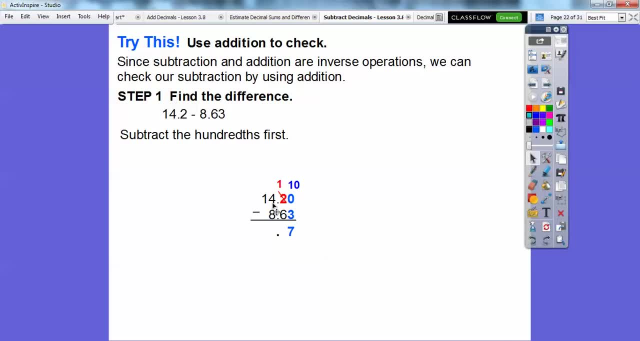 borrow from this four ones right here, so four ones will become three ones, and this will become eleven tenths, because we'll add ten to that. okay, all right. so here we go, and then, when we borrow, there's our eleven ten, so we can do a total of eleven tenths minus six tenths is five tens right there, and then we're. 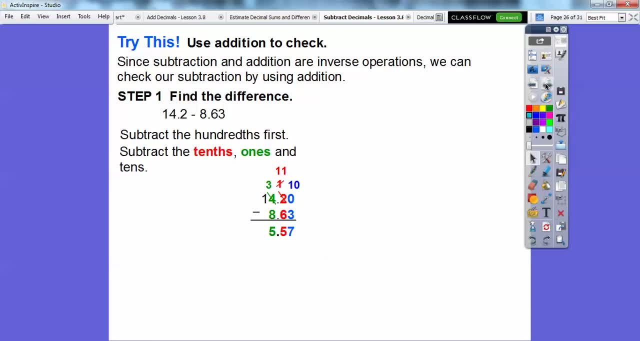 left with thirteen minus eight. thirteen minus eight gets us five, right there, okay. so let's, let's check our answer here. we'll, we'll add the difference to the number. so here's the difference. right here, we'll add the difference to the number. we subtracted. so we subtracted this. so this five point five. 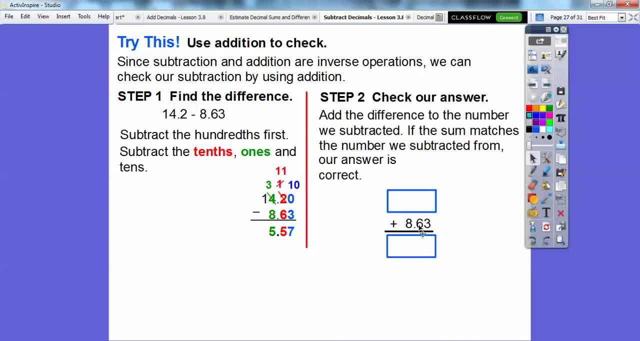 seven is going to go up here, and if the sum matches our, our original number right here, fourteen point twenty- then we did it correctly right here. so let's go ahead and put the five point five, seven in there and let's go ahead and add: okay, so seven plus three is ten. we'll put a zero here and carry. regroup the the one. 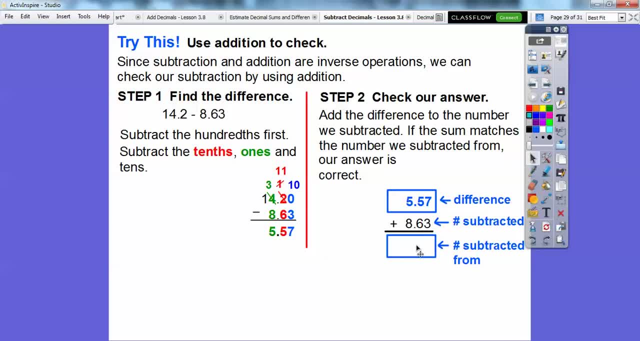 right up there. so one plus five would be six plus six would be twelve. so a two would go right there and we'll regroup and put the one right there. okay, one plus five is six, and six plus eight is that fourteen right there. so so it does.